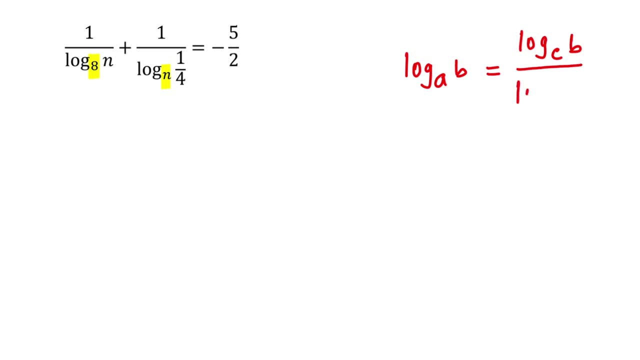 the same thing as log base c of b divided by log base c of a. c is now a new base and it can be any number as long as it is greater than 0 and different from 1.. This is from the definition of logarithm, Because it is possible to write both 8 and 1. fourth, as a power of 2, you can choose 2. 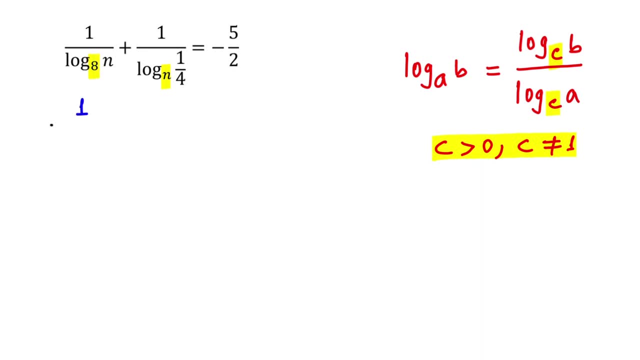 as a new common base. So you can rewrite log base 8 of n as log base 2 of n, divided by log base 2 of 8, and you can rewrite log base n of 1, fourth as log base 2 of 1, fourth, divided by log base 2 of n. 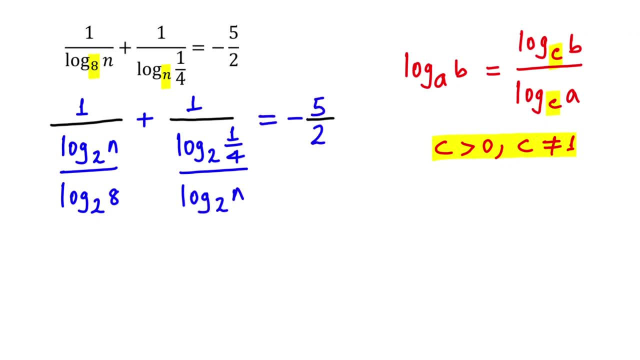 To divide a whole number by a fraction. you can multiply the whole number by the reciprocal of the fraction, right? So this is the same as log base 2 of 8 divided by log base 2 of n. and this is the same as log base 2 of n divided by log base 2 of 1. fourth, Alright, now let's evaluate log base. 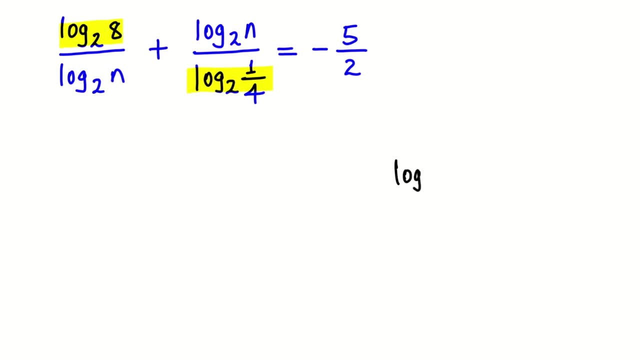 2 of 8 and log base 2 of 1. fourth, 8 is the same as 2 to the power of 3, right From the power property of logarithm. If you have log base a of m to the power of p, it is the same as p times log base a of m. We just 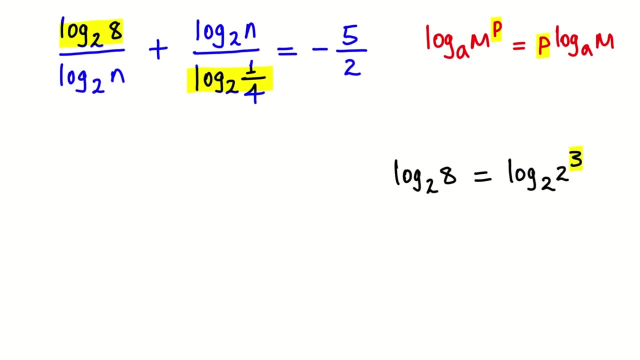 moved the exponent of the argument in front of the logarithm, So likewise you can move 3 in front of the logarithm. If the base and the input of a logarithm are the same, then the logarithm equals 1.. So similarly, log base 2 of 2 equals 1, and 3 times 1 is 3.. So in the equation you can replace: 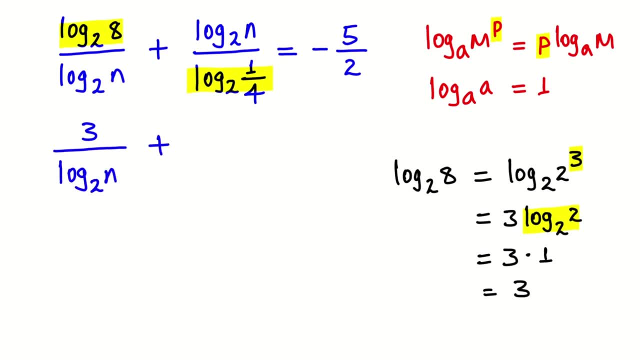 log base 2 of 8 with 3.. Let's evaluate now log base 2 of 1 fourth. 1 fourth is the same as 2 to the power of negative 2. right, Using the power property of logarithm, you can move negative 2 in front of the logarithm. 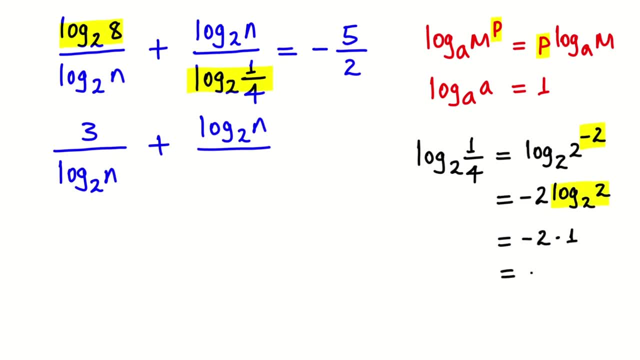 Log base 2 of 2 equals 1 and negative 2 times. 1 is negative 2. So in the equation you can replace log base 2 of 1, fourth, with negative 2.. Now let log base 2 of n equals some variable. 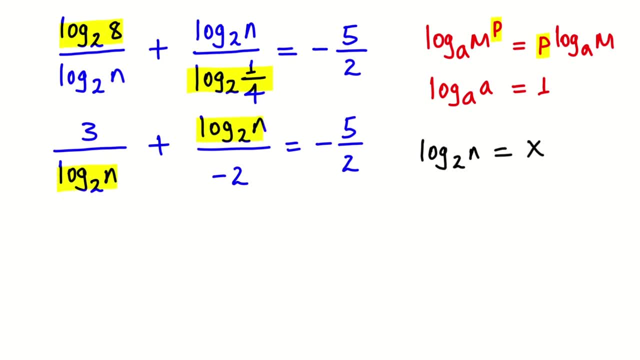 And replace log base 2 of n with x in the equation. So you're gonna have 3 over x plus x over negative. 2 equals negative 5 over 2.. Okay, now get rid of the fractions by multiplying both sides of the equation. 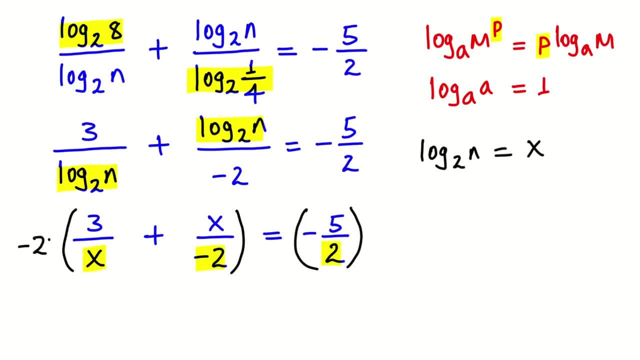 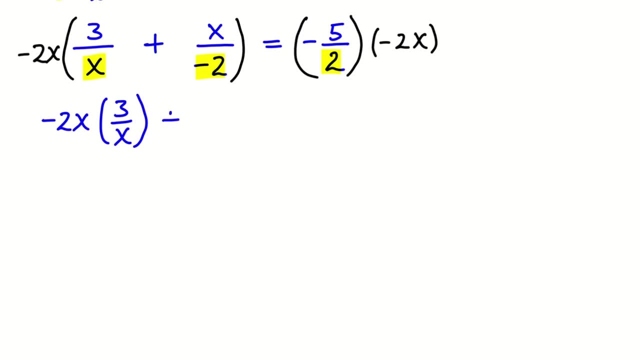 by the LCM of the denominators. The LCM of the denominators is negative: 2x right Distribute negative 2x Negative 2x times 3 over x plus negative, 2x times x over negative 2.. 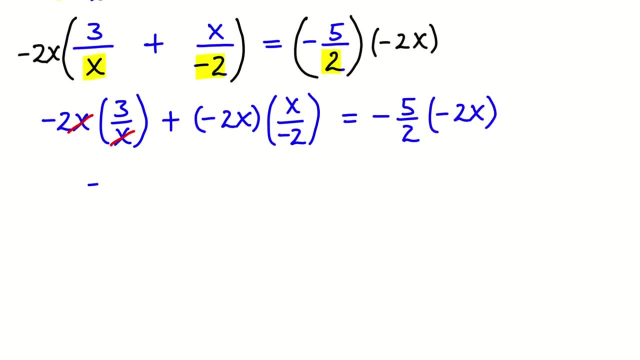 You can cancel the x's and negative 2 times 3 is negative 6.. You can cancel the negative 2's and x times x is x squared. You can cancel the 2's and negative 5 times negative. x is 5x. Now move negative. 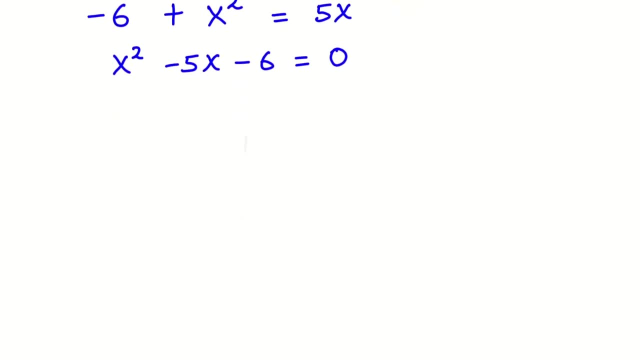 5x to the left side of the equation. Let's solve now this quadratic equation using factorization method. For that, find two numbers whose sum is negative 5, and whose product is negative 6. What do you think? these two numbers are Negative- 6 and 1, right? 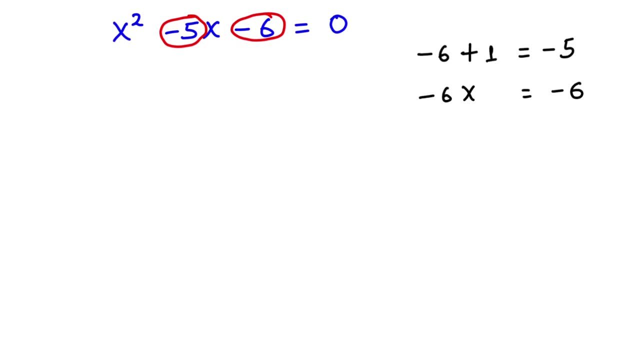 Negative 6 plus 1 is 5. And negative 6 times 1 is negative 6.. So when you factor this quadratic equation, it becomes x minus 6 times x plus 1.. Using the zero product property for this product to be 0, either x minus 6 should be 0 or x plus 1 should be 0. From this, x equals 6 or x equals. 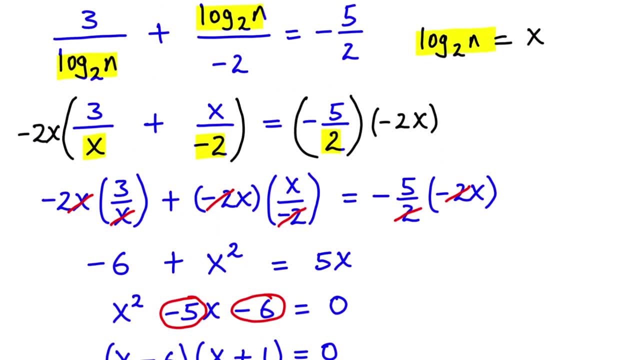 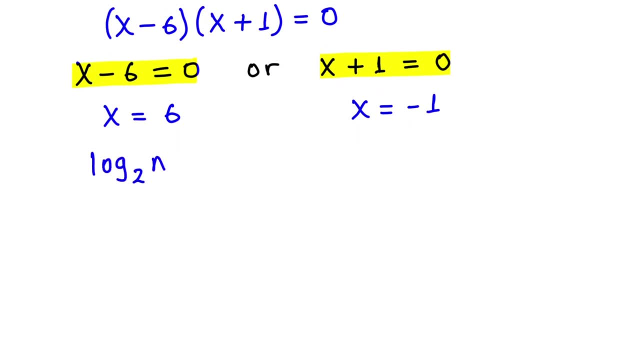 negative 1.. If you remember, we said that log base 2 of n equals x right. So when x equals 6, you have log base 2 of n equals 6.. When x equals negative 1, you have log base 2 of. 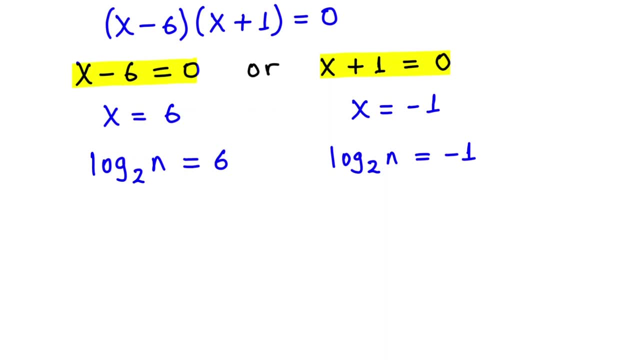 n equals negative 1.. Now convert these logarithmic equations to exponential form. This is equivalent to 2 to the power of 6, equals n, And this is equivalent to 2 to the power of negative. 1 equals n, 2 to the power of 6 is 64 right And 2 to the power of 6 is 64 right And 2 to the.